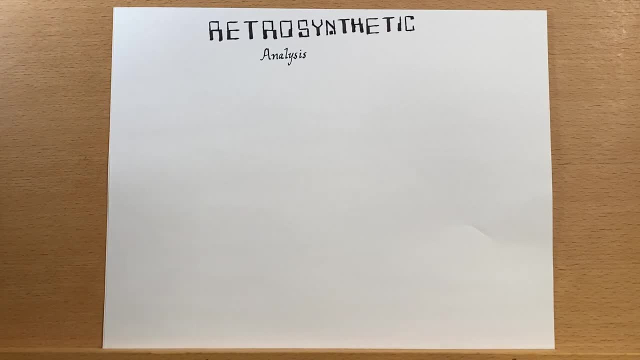 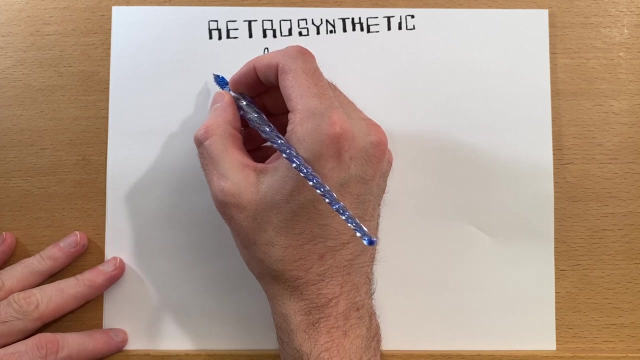 Let's examine a strategy that we can use to look at a complicated synthetic pathway. This is retrosynthetic analysis and it may seem counterintuitive at first, but if we start at the product then we may have an easier time finding out how to synthesize it. So let's say, for example- and we'll just do an example- to 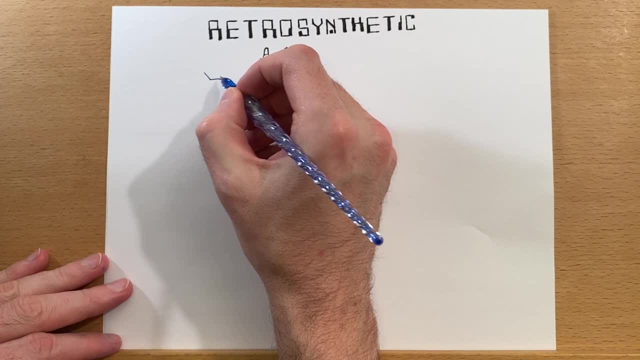 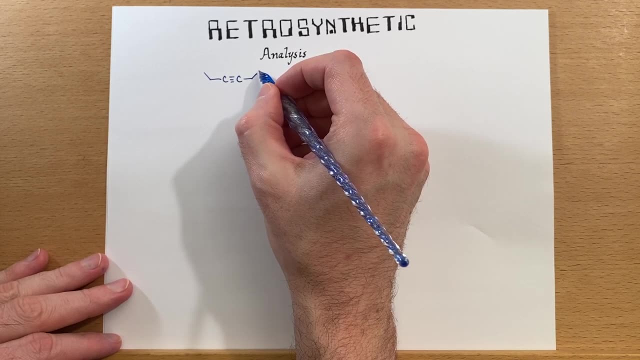 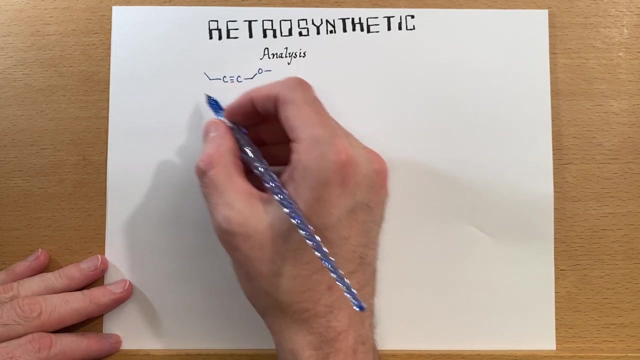 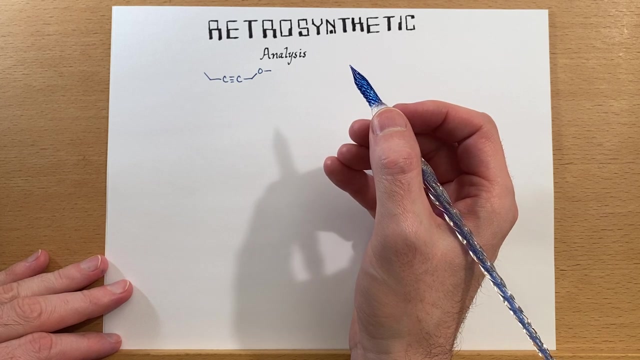 talk about how this can work. we would like to make this molecule, and let's also say that, while we would like to make this, we're only going to allow ourselves to reagents that have three or less carbon atoms in them, So we're going to have to break this apart. 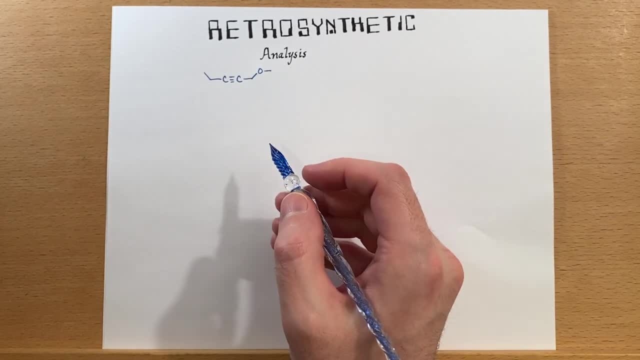 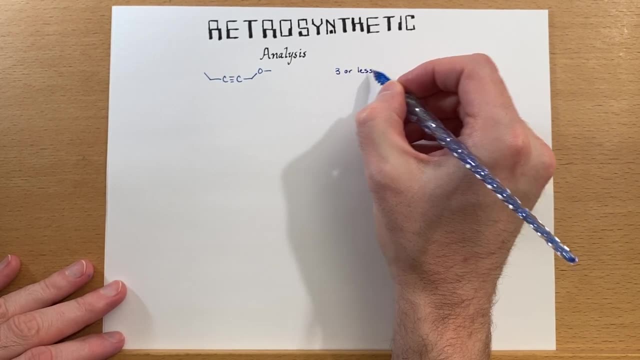 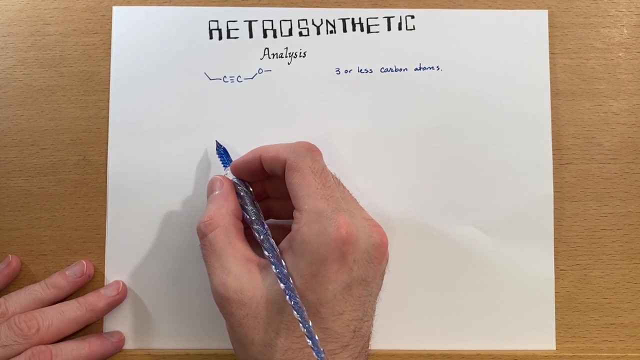 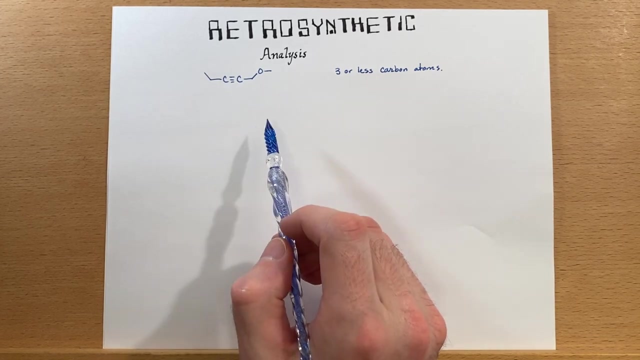 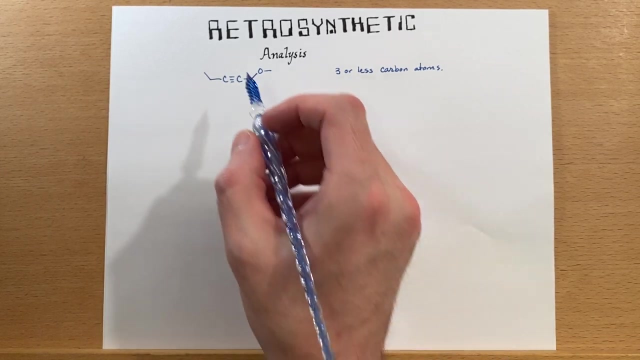 into several pieces in order to make it. if we're limiting ourselves that way, Okay. Now, the way this works is we start looking for places where we could break this molecule apart and then think about reactions that we could use to put together, put this molecule together. 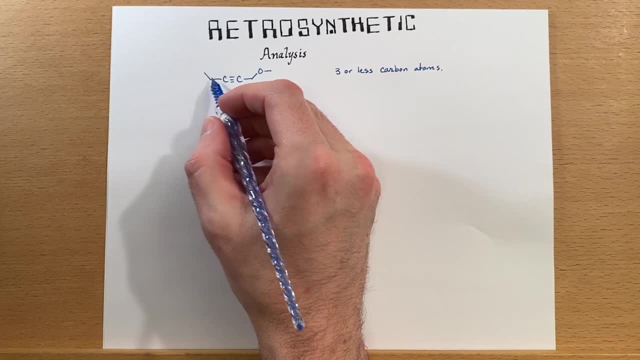 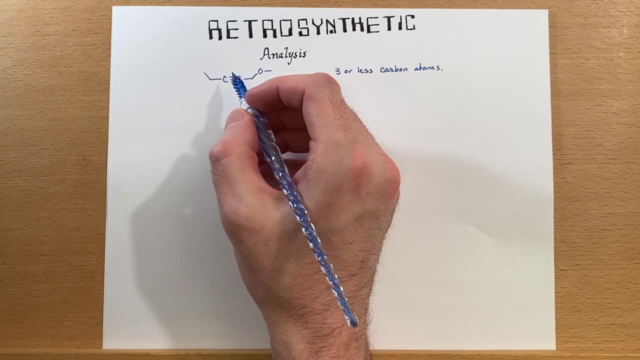 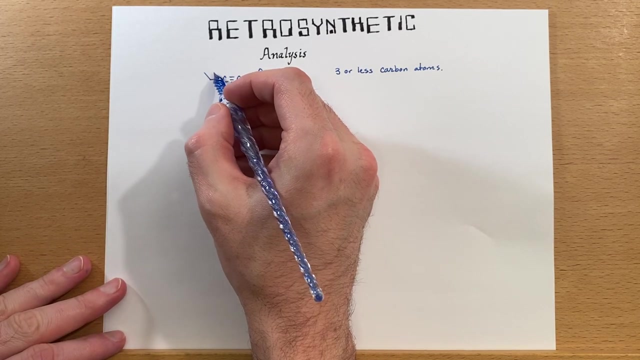 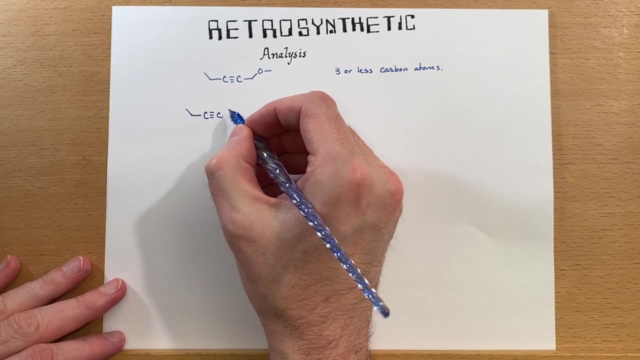 So one of the options would be looking at where the functional groups are and deciding we could break it at one of the functional groups. So let's try to see what would happen if we break this bond right here. So the way that we start to draw this out, we'll draw this molecule. 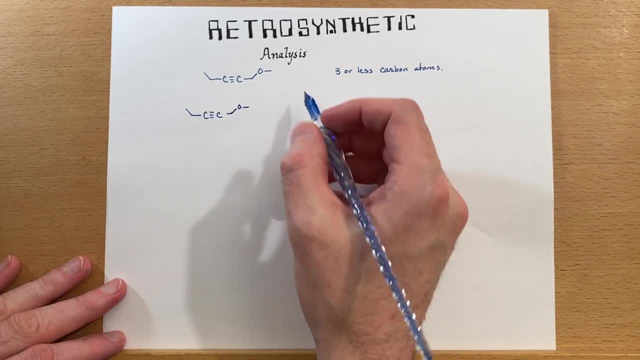 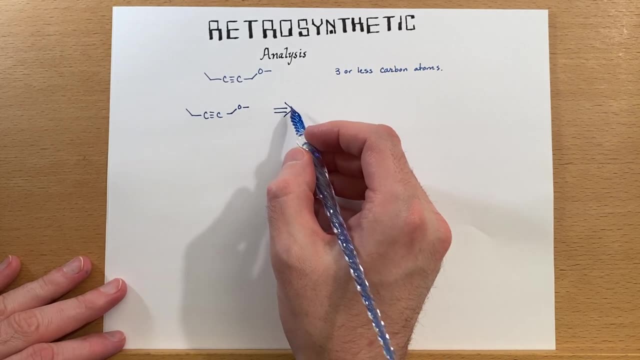 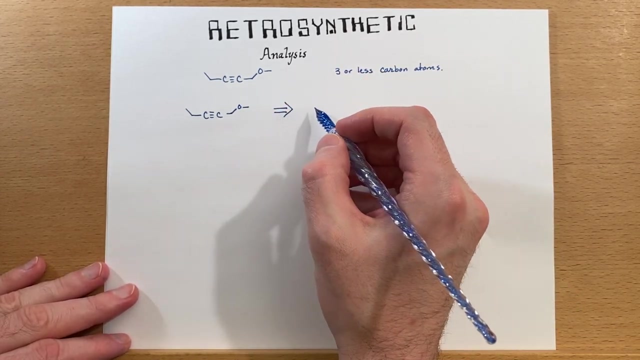 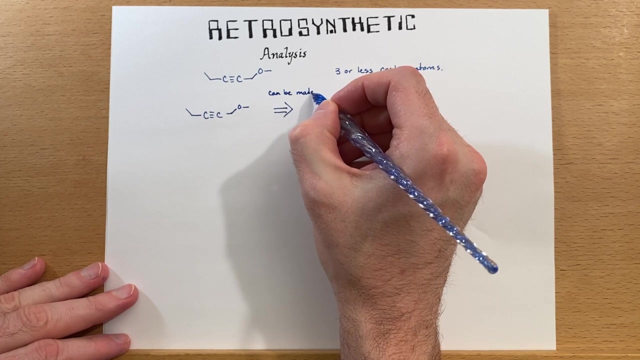 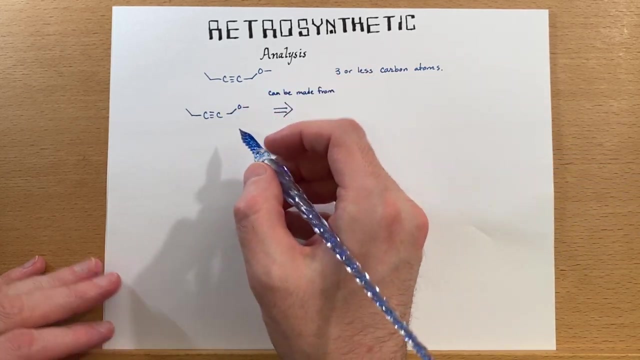 and then we'll draw a, a retrosynthetic arrow, which is just an arrow that has a couple of lines in it. It's kind of a more open arrow, And the way you would read this is can be made from: So in reality, the reaction is going to go this way, but we're trying to break this apart. 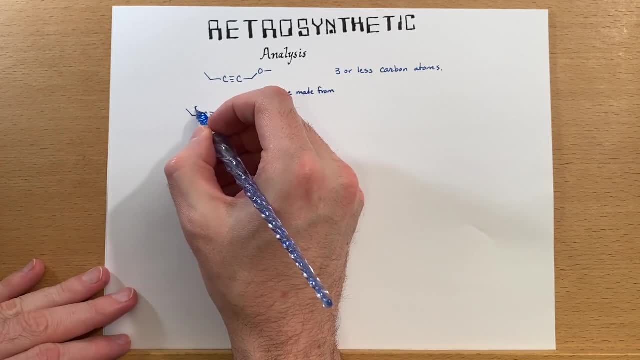 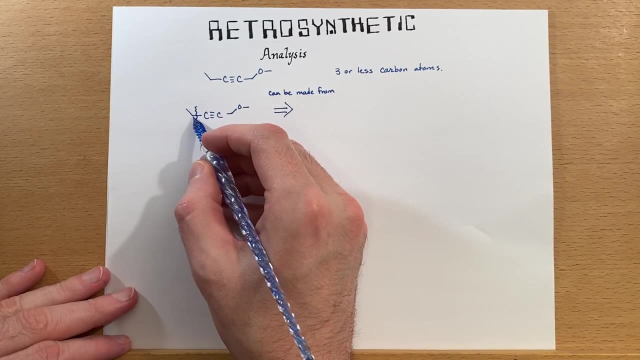 So we're going to draw a a retrosynthetic arrow into more manageable pieces. So let's see what would happen if we break this bond right here. If we did that, we could have a two carbon piece here and then a one, two, three, four carbon piece there. 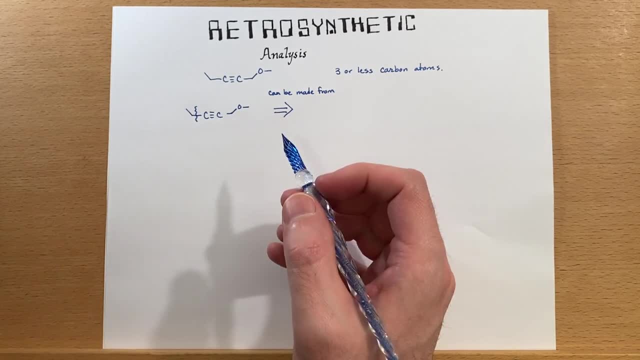 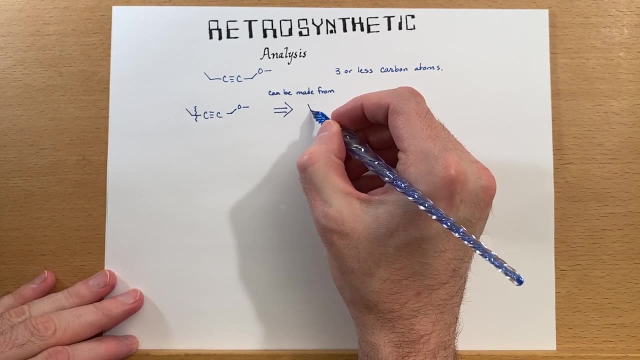 So we'll. we'll still have some breaking apart to do, but we'll be closer to what we need, which is the three carbons or less that we just arbitrarily decided for this exercise. So we need some kind of leaving group over here. 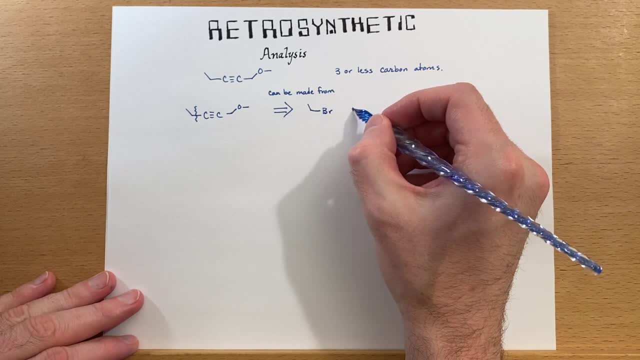 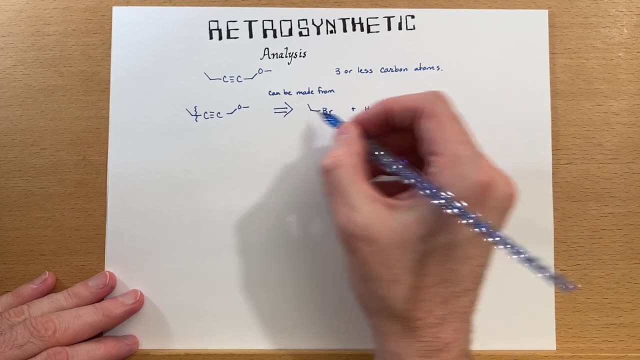 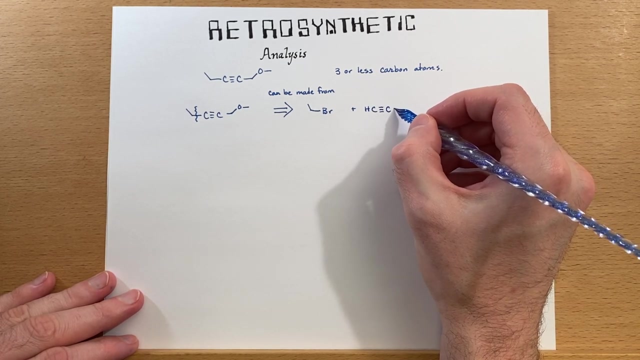 So we'll just stick with a bromine here, And then we've got our, the other molecule that we have here, which is still too many carbons. but this part is only two carbons, So we're getting closer. So now that we have that, 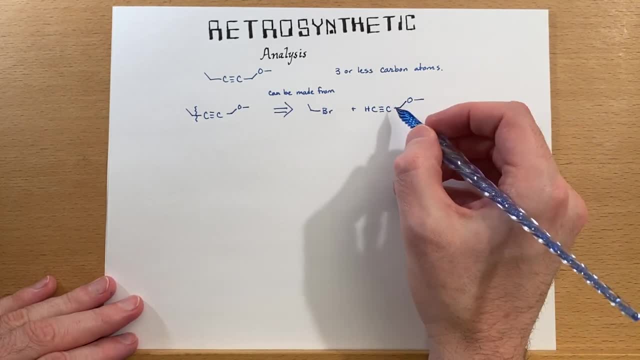 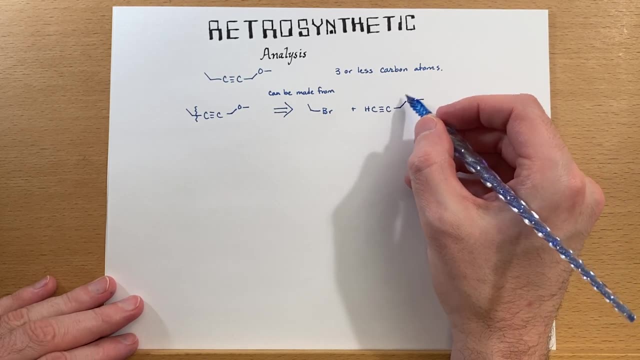 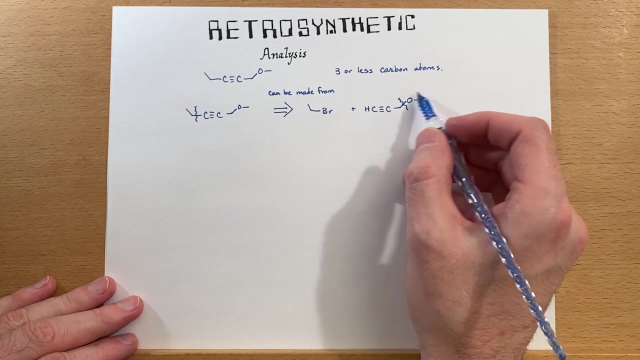 we'll usually look for another place of another functional group location that we could break this molecule apart at. So here's a good spot right here, And that will get us down to one, two, three carbons there. This only has one carbon and we have reactions that can make ethers. 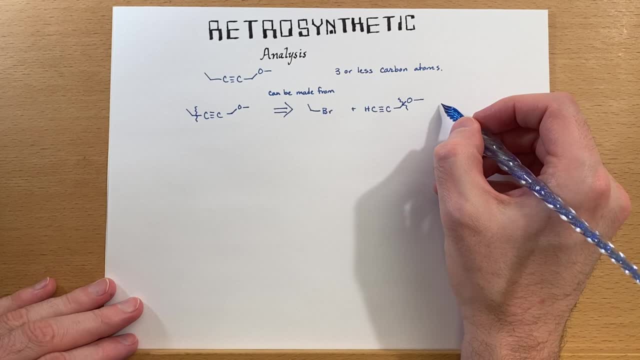 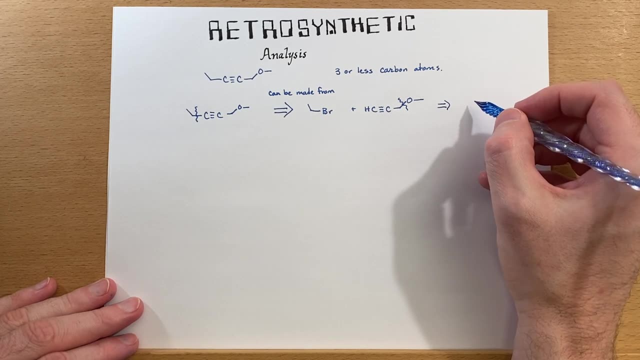 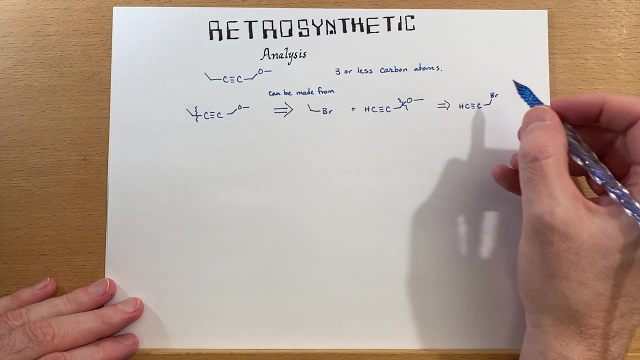 And so let's just continue drawing in this way. We'll ignore that part right there. but now So we've got a leaving group added onto there and we're just gonna stick with bromines just because it's convenient. And then we need the alkoxide. 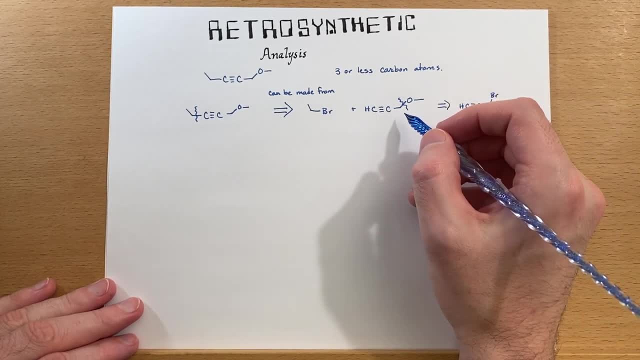 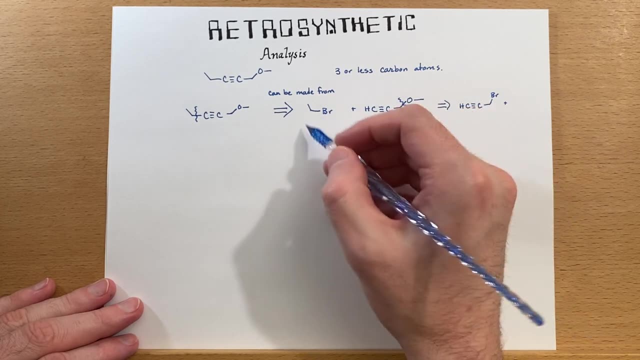 We're gonna do Williamson ether synthesis here, And in this case we're going to deprotonate this alkyne and then use that to make a carbon nucleophile, And then we'll click this button here to do that. Now we're gonna get the solution. 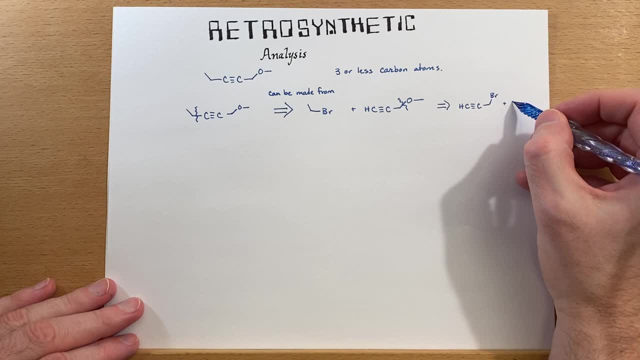 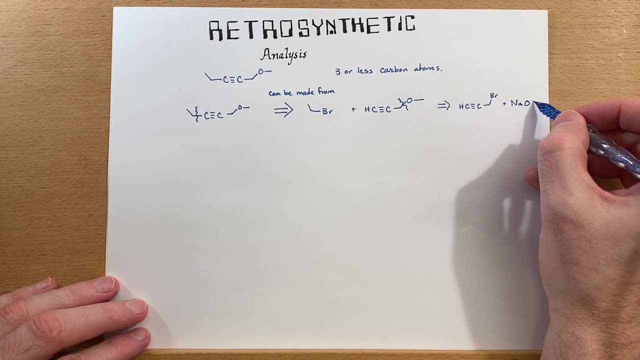 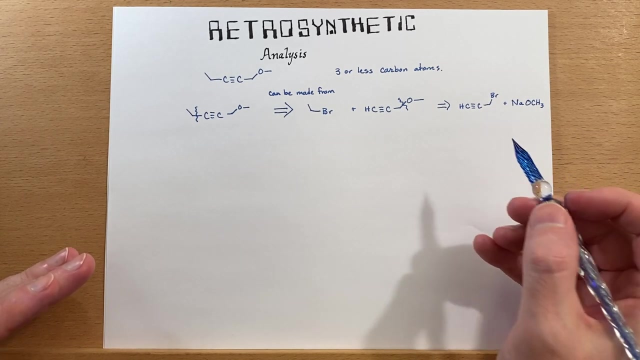 an attack there, right? so sometimes we don't have to think as much about how what reagents we're going to use right away. if we have that in mind, that's great, because we might end up in a dead end location where we just can't go. 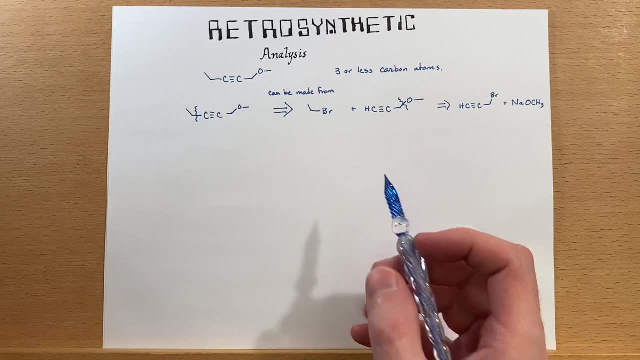 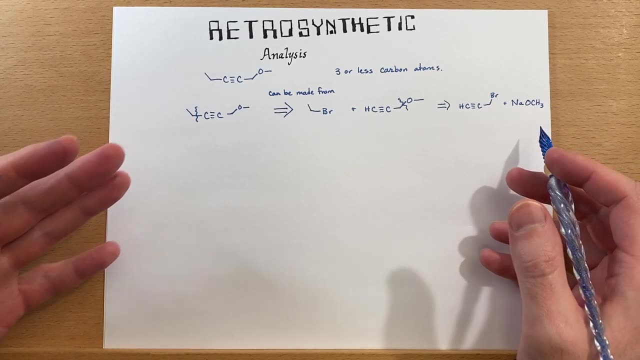 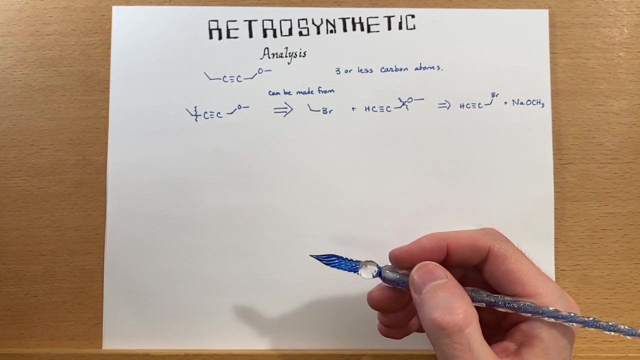 forward, we'll have to try breaking another bond and instead of that direction. so once we've conducted the retrosynthetic analysis, then what we'll do is we'll turn around and we'll go in the forward direction and we'll write down all the conditions and we'll really check to make sure that the selectivity 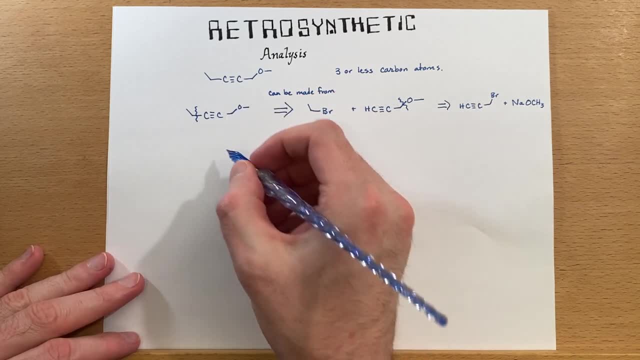 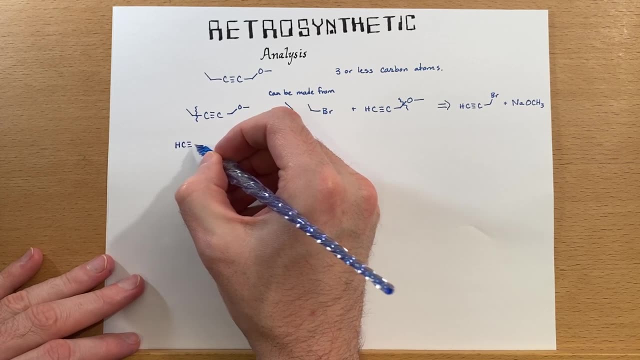 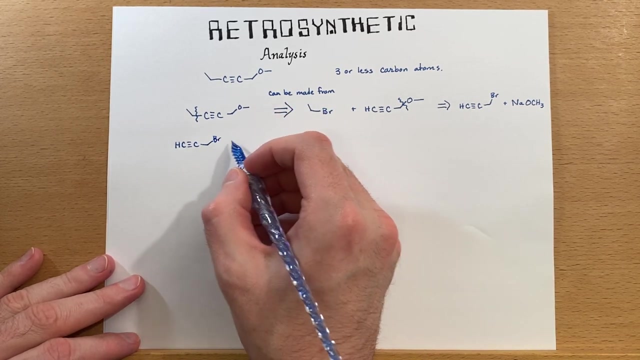 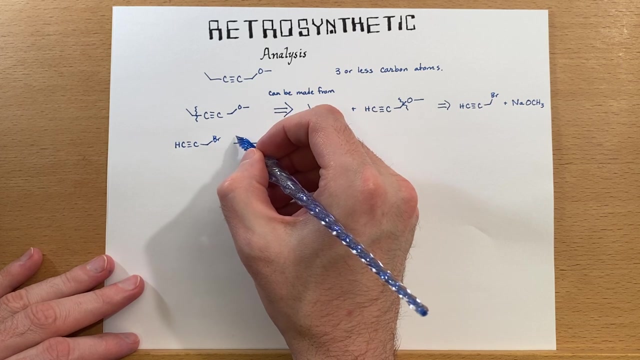 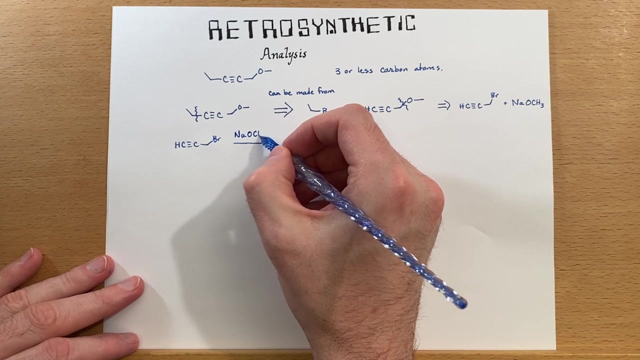 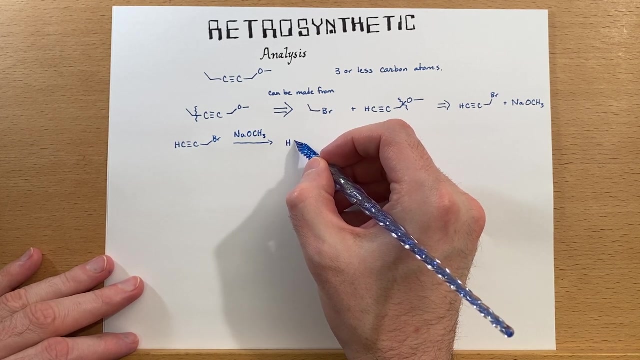 is what we need and we are actually going to make the product that we want. so we'll do that now, starting with the ether synthesis. and the nice thing about ethers is, once we add it on to the molecule, generally the functional group is quite tolerant of other transformations, other conditions. so now we've made our intermediate here. 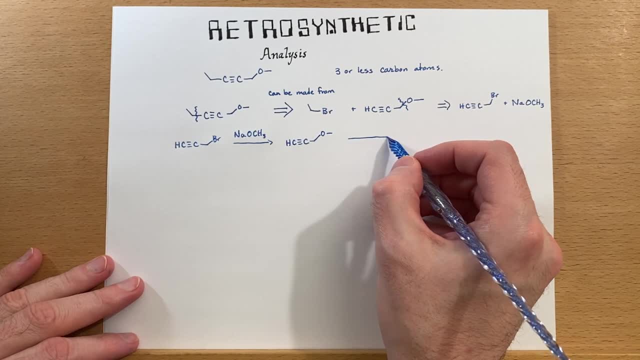 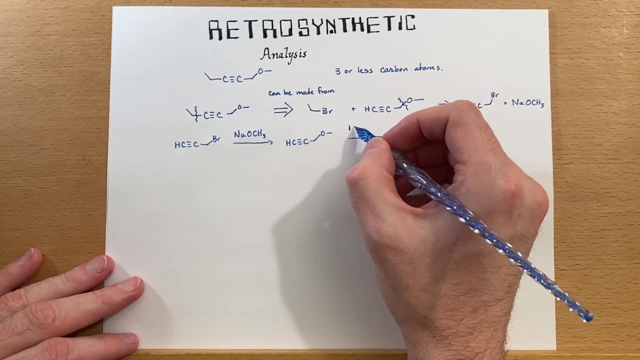 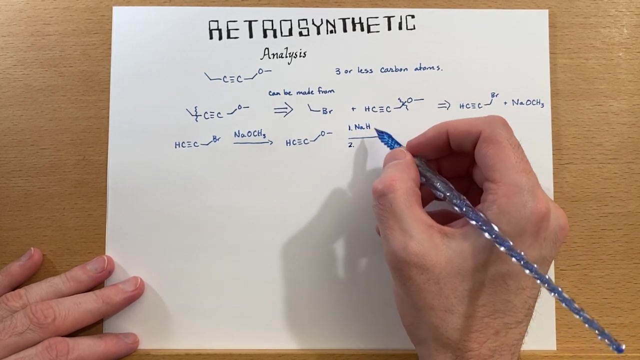 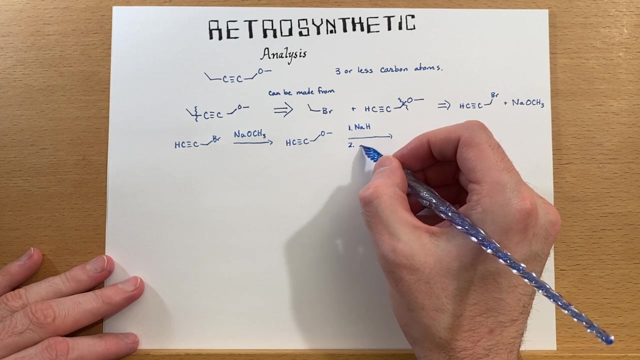 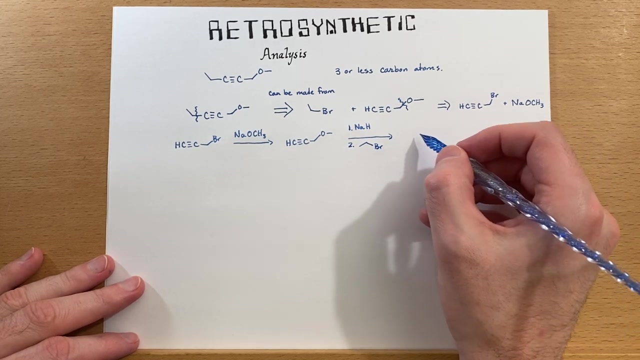 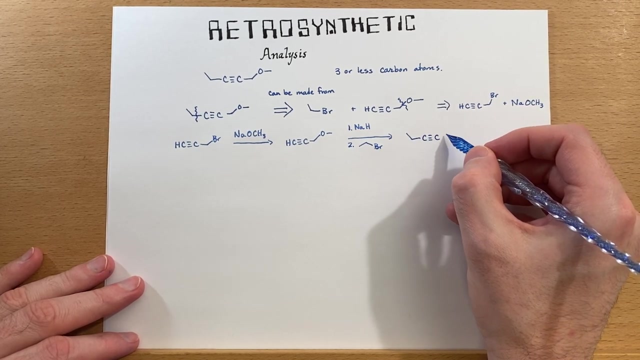 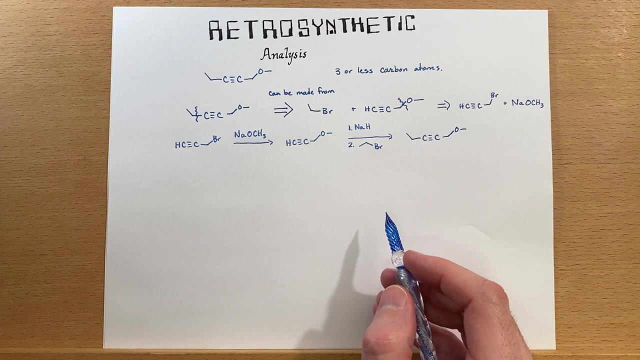 at this point we can form the carbon nucleophile. we can pick sodium hydride or a similarly strong base, and then we'll add our bromoethane, which will then affect the product that we were looking for in the first place. now, this is one option for making this molecule, but there is more than one way. 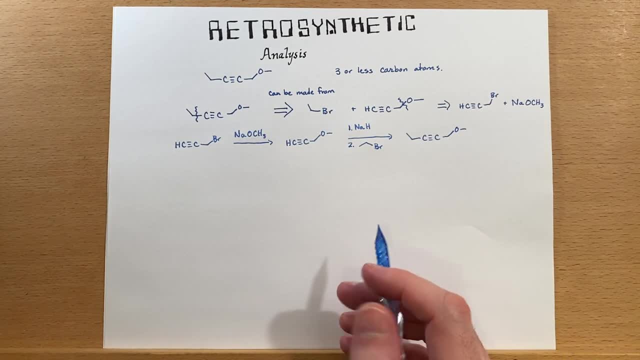 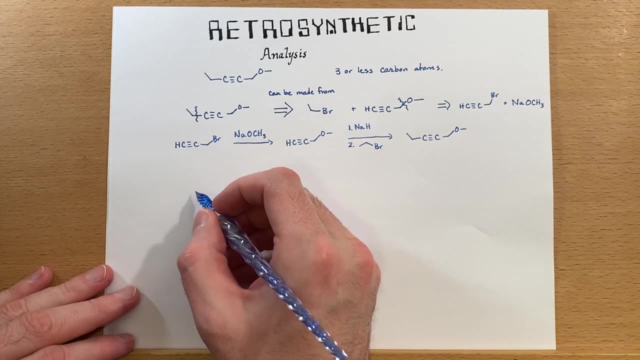 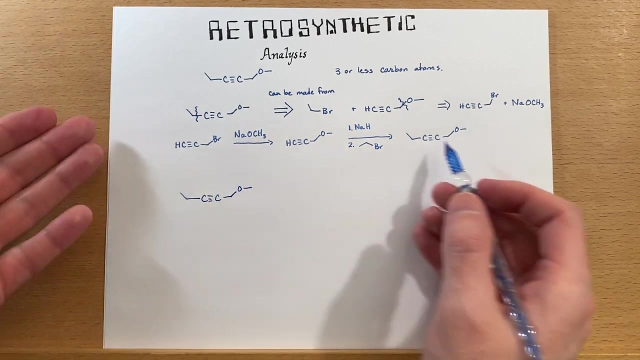 to usually conduct us in a synthesis, especially when it gets to be complicated. now there's ways that we could use to decide which ones would be better, but let's look at this for now, so let's examine another way to do it. that could be possible. now there could be problems with this way. there could be problems. 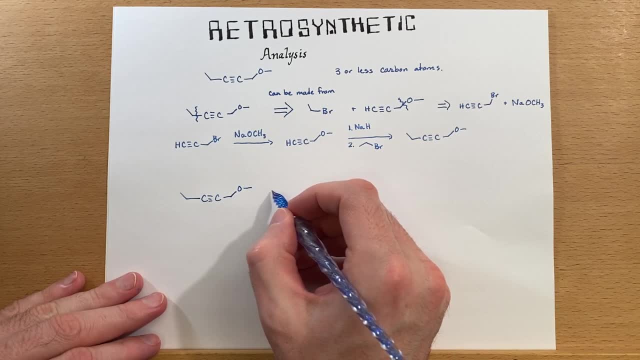 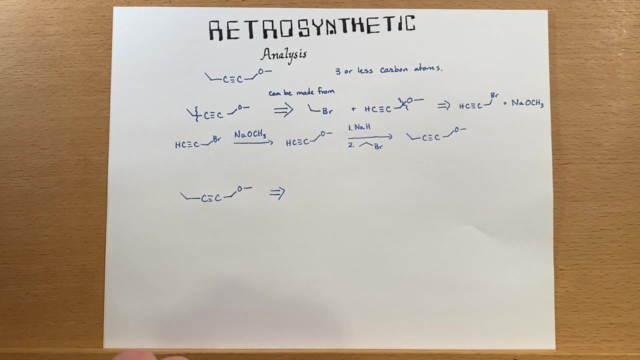 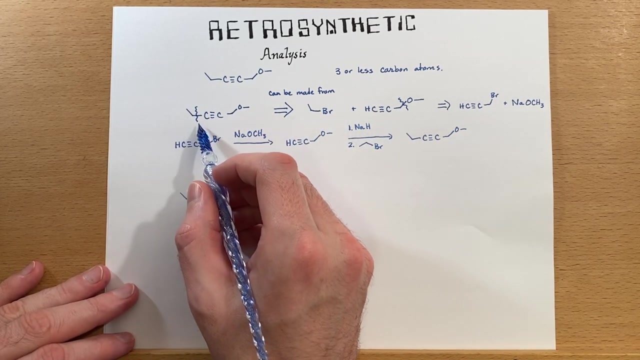 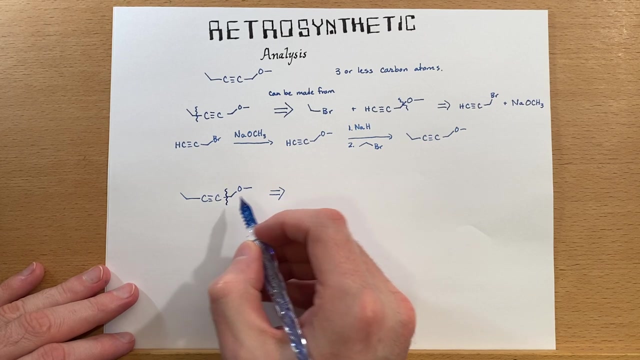 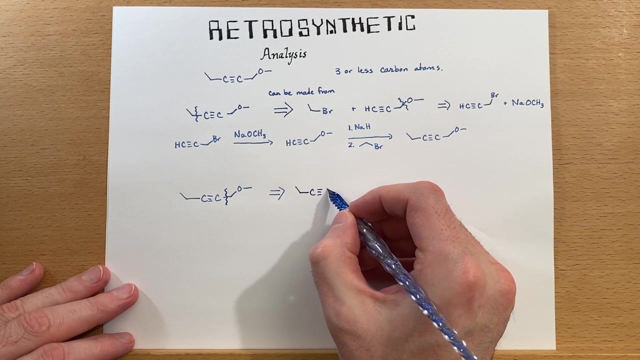 with the other way. we'll have to look at that at some point, certainly hopefully before we do it in the lab. all right, so this time we broke this bond right here. instead, what if we broke this one? so a break right there, and then we'll just imagine that we're going to turn this into a nucleophile carbon. nucleophile. 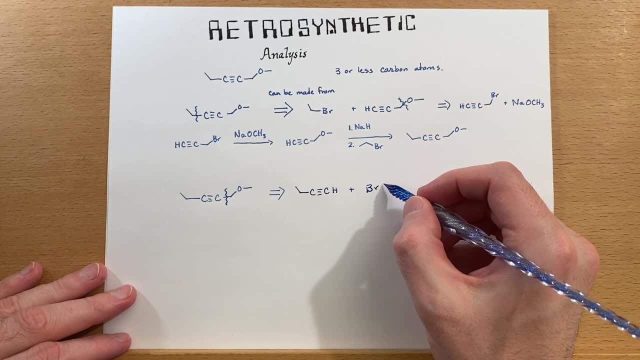 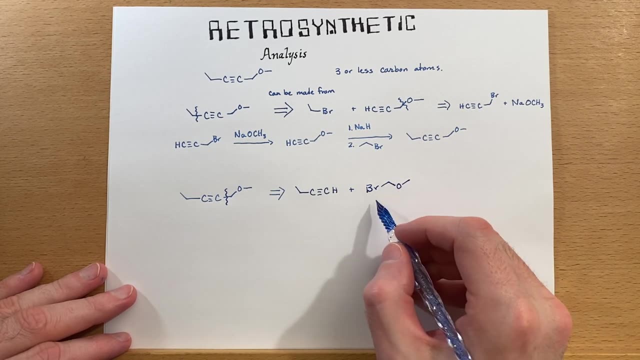 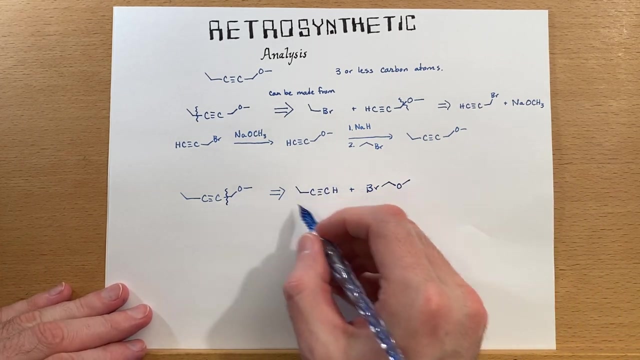 so we'll just put a leaving group over on the other molecule. this only has two carbons in it, so we're we're good on that one. this one has one, two, three, four, so by our own rules we're going to have to break this part a little bit more. 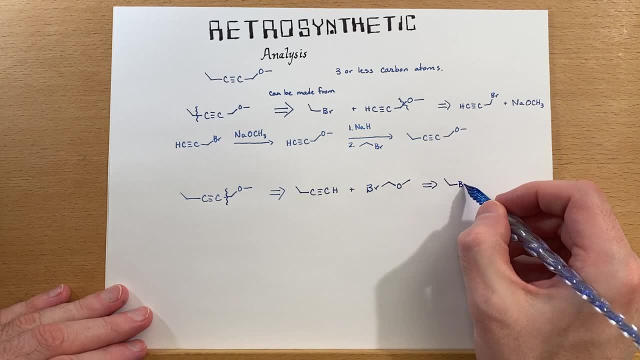 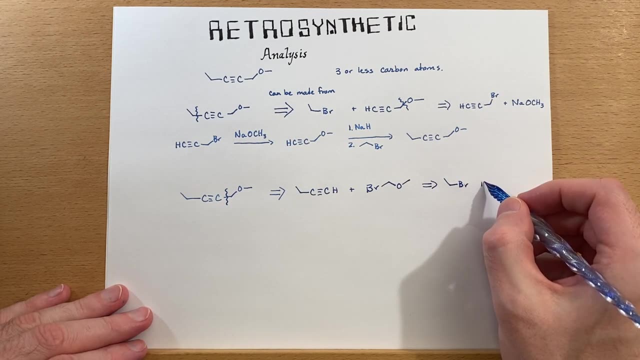 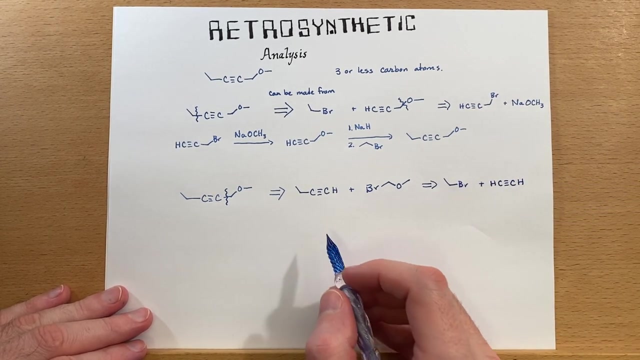 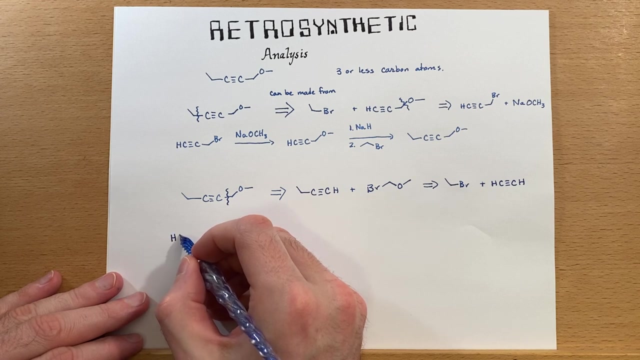 so we could say that could be made from the bromoethane and let's just say acetylene. and so if we wanted to write this in the forward direction, we would do this again. we're going to use the sodium hydride. that's an h and an i. 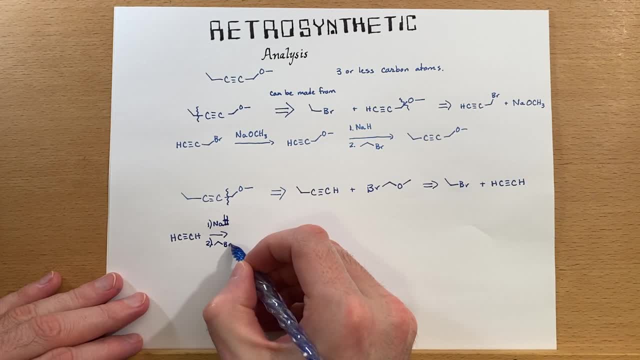 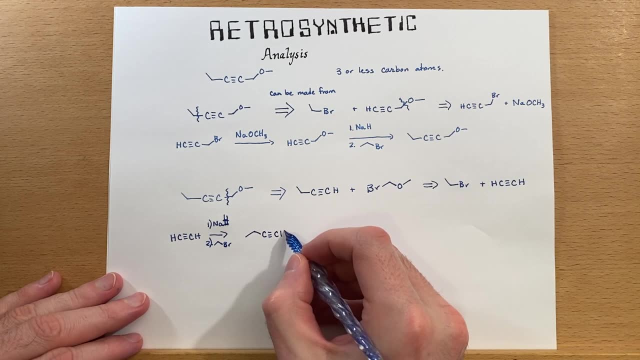 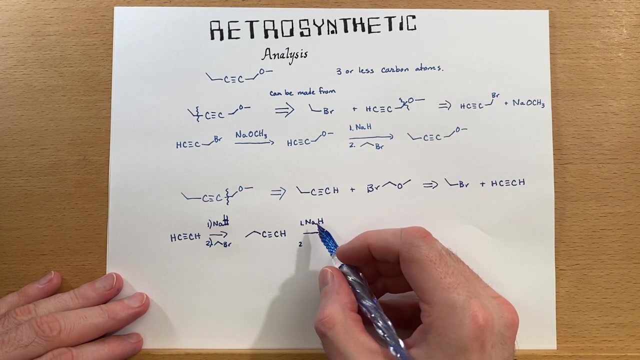 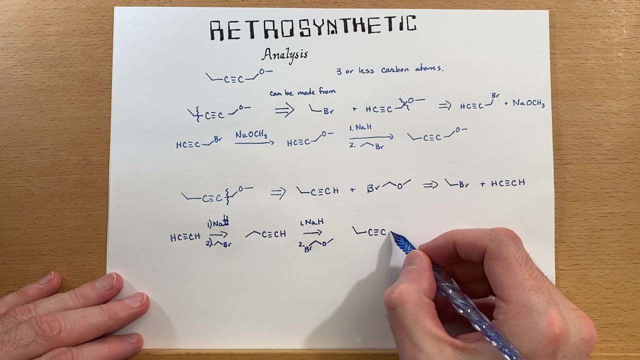 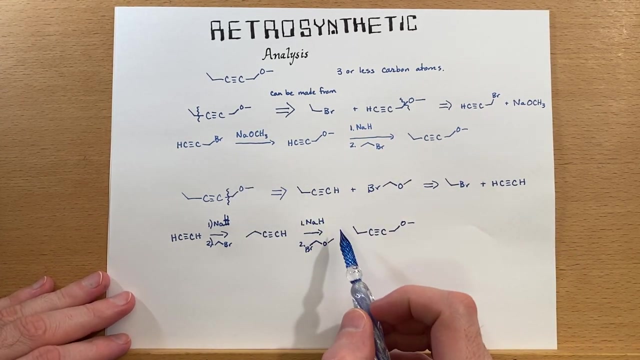 and our bromoethane. we should be able to make this, and then we'll just form our carbon nucleophile again- same kind of reagents, only now we're going to change to a different substrate and we could affect our product. now i would argue that the first synthesis is a little bit better.